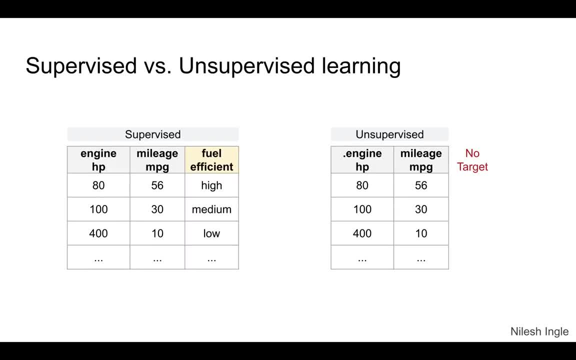 What is the population and what is Gaussian distribution. So here is an example. on the left hand side, we have a data set which has two features, which is engine horsepower and mileage in miles per gallon, And the target here is categorical and we have a target that tells if each of those vehicles, if it's, if it has high fuel. 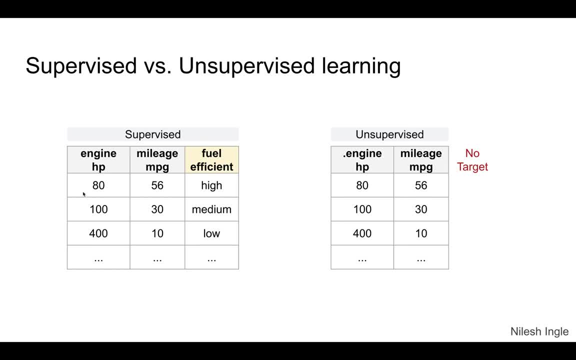 fuel efficiency or low fuel efficiency and, for example, first vehicle in that is represented here in the first row has high fuel efficiency, second one has medium, last third one has low. now we have seen that when we train with supervised learning methods, we input both the features as well as targets. so 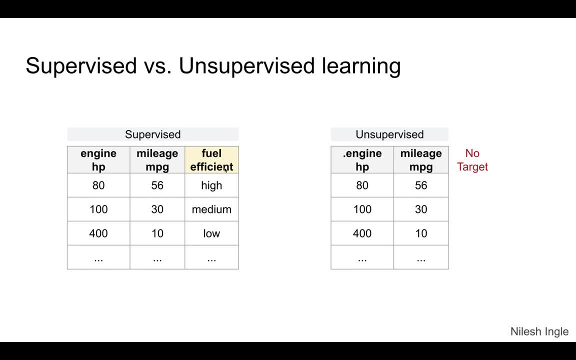 this is represented as X train and this is our Y train that we input to the fit method when performing the fit and then test method also has sorry. the test data also has both the mean, sorry. it also has the features and the target, so we use that target to get the final scores or to see the results. 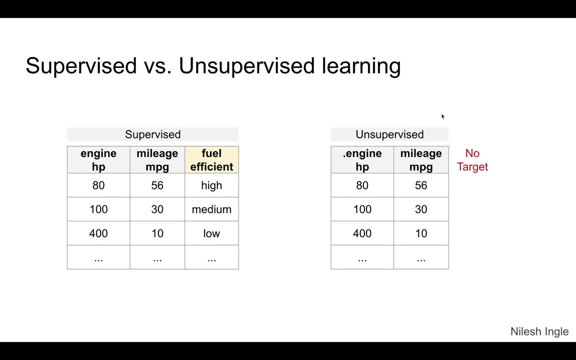 how the model fits with the unseen data. Now, in case of unsupervised learning, we do not have the target, so the data would simply be engine horsepower and miles per gallon. So the task that we are going to look at in this video pertains to 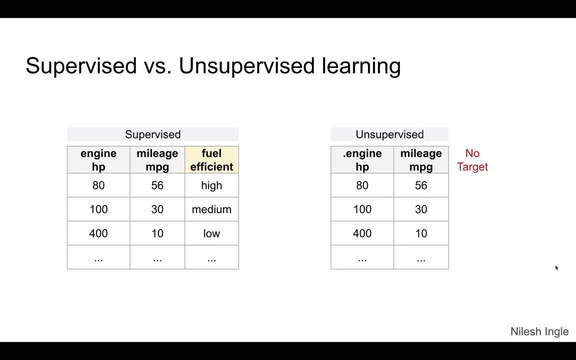 finding groups. so if we try to plot this data on a two-dimensional plot with maybe engine horsepower on the x-axis, miles per gallon on the y axis, then we may able to. we may be able to see three different groups of points clustered together, And so unsupervised learning method can help us identify those groups. 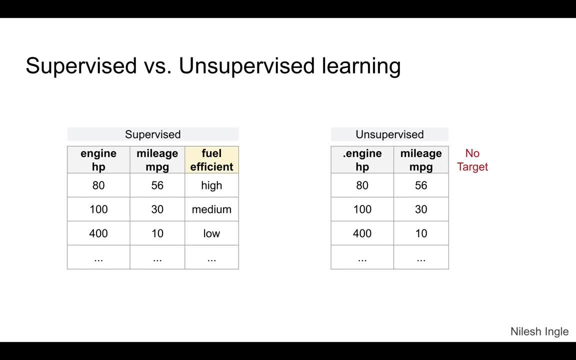 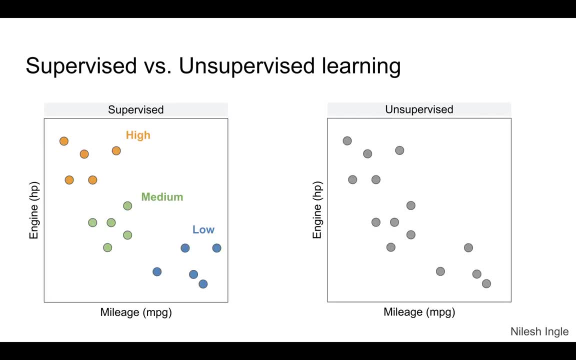 of points. groups of points can help us identify those groups of points. In this case we want to groups of points. In this case we want to data points and then we can label them as high, medium or low or any other labels. so here we can see that the orange, green and blue are the three. 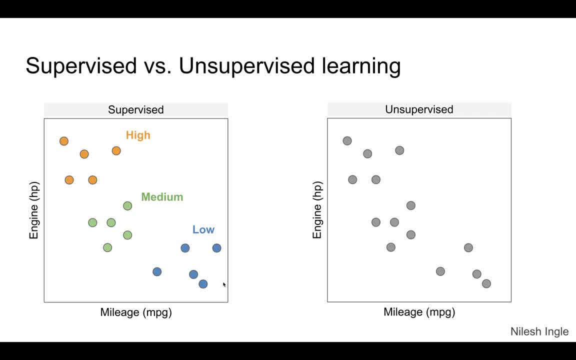 groups that are already labeled in the data set when we are, when we you want to use them for the training purposes. however, in case of unsupervised learning, the data is not labeled. however, we do see these clusters, and so we use the distances from these data points to see which points belong to. 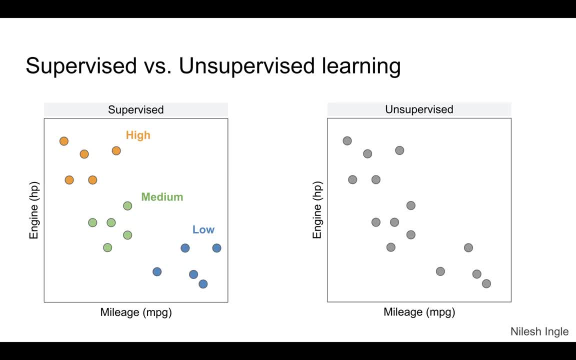 which clusters and we'll look at how that is done in more in-depth in future slides. so with supervised we we have the target, so we know the groups there. in unsupervised we call them clusters of data points and we can identify cluster 1, cluster 2, cluster 3, as shown here, and then those are labeled for us if we want. 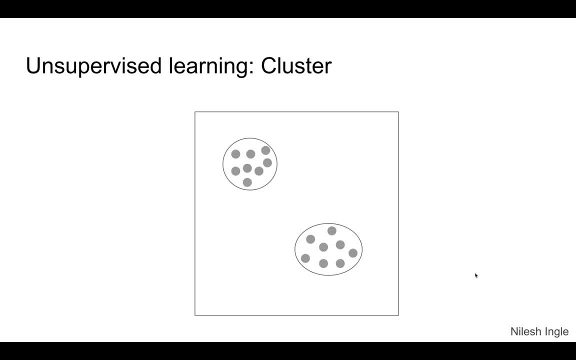 to do further processing. the clusters or groups can be of different structures. here we have two well separated groups and they look like- looks like they are and have kind of similar density of data points. so the spacing between the data points is more or less same in both the clusters. 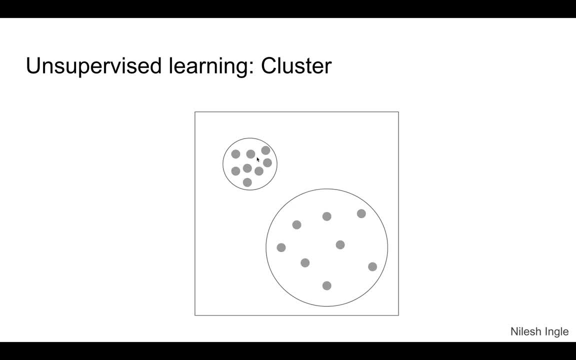 in this cluster. they are well separated, but then the density or distance between the data points within each of those clusters is different. these are more compact, these are spread out. now this is another version in which we can see that the smaller cluster is within the outer group, which is more spread out. so that's another. 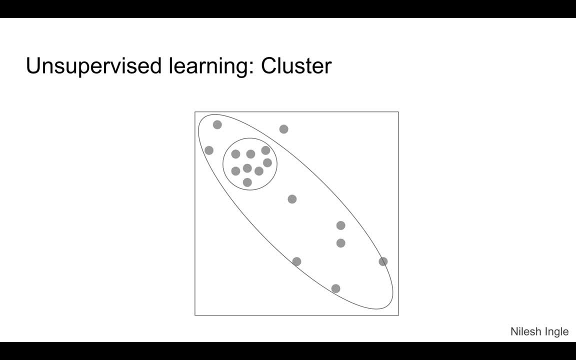 type of data. we can help find clusters using unsupervised learning methods, and these are two overlapping dense clusters, and. And then we have this cluster, which is interesting and complicated but, as we'll see, Gaussian method- mixture models can help us find these two clusters based on the probability values. 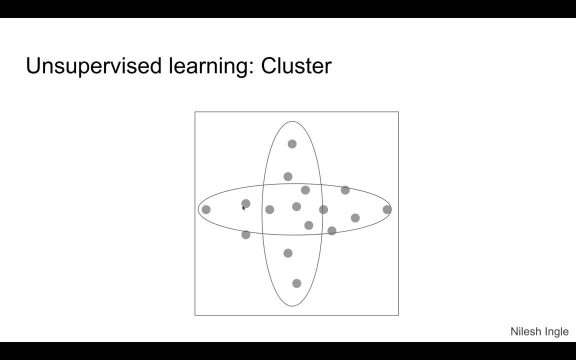 of each of these data points and how they belong to that particular cluster. Here is another set of structure of data where we have these arranged in this fashion, And these are just a few examples. There are, I will say, maybe as many structures you could find, as many. there are data sets. 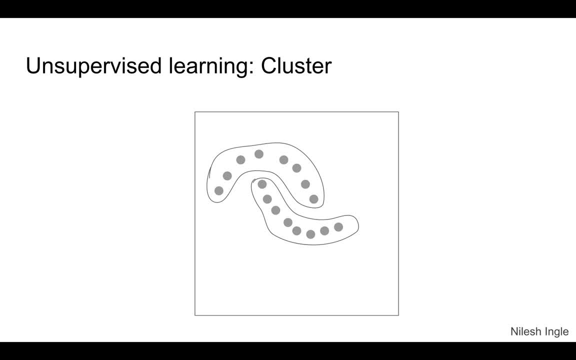 So this is just to give you an intuition of data, What type of structures we can find in data sets when we are performing unsupervised learning to find clusters. So why then, is unsupervised learning used? So first is, as we looked earlier, it can help us understand the structure of data. 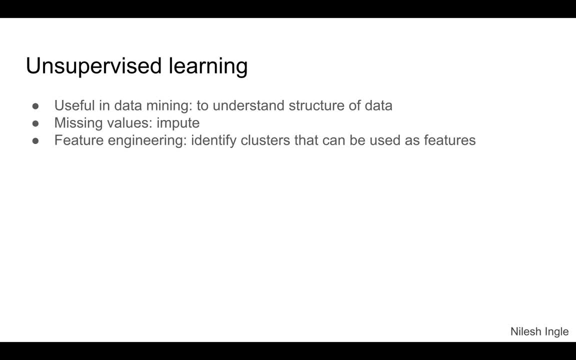 It is also used to impute missing values. So let's say, for example, if we have a cluster of data points in which we have values for five out of 10 features, But we know that countries that particular data point belongs to that particular cluster. 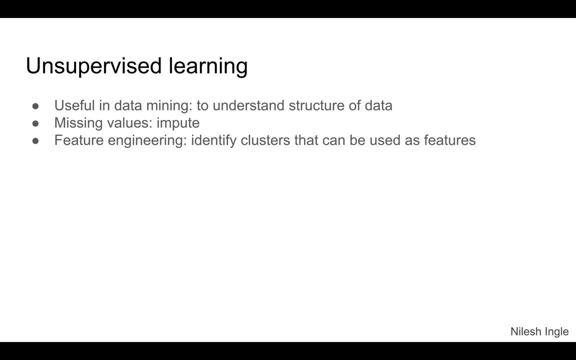 Then we could assign values within that cluster to that data point. So we can use an operation as the members to get these values based on the songty DEMO data point which has missing values. so out of five we can add maybe, or the remaining five values for the features to that data point. feature engineering is another application, so 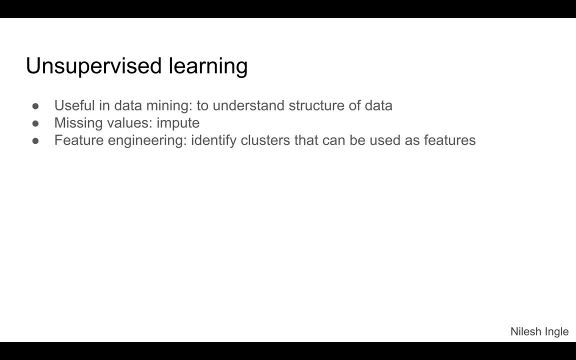 let's say you have a data on customers who shop in a grocery store and, depending on their monthly spending on groceries in that store, we can segment them based on high spender, low spender, medium spender and accordingly, the marketing team could use that information to provide maybe discount coupons or new products to each of these customers. 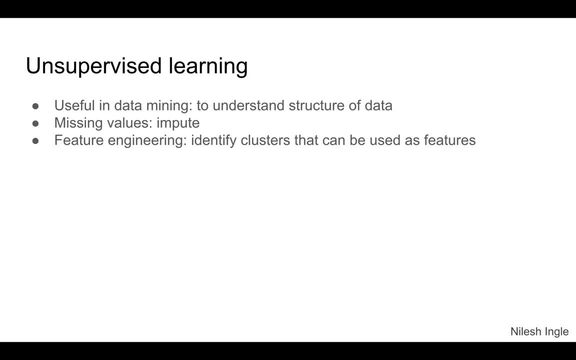 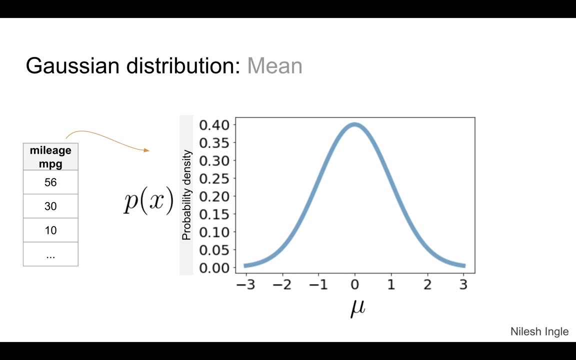 so segmentation- market segmentation- could be one of the uses of this feature engineering. now let's switch gears a little bit and talk about Gaussian distribution. so you've probably seen this curve several times. if you have not, this is a quick refresher on that. let's say we 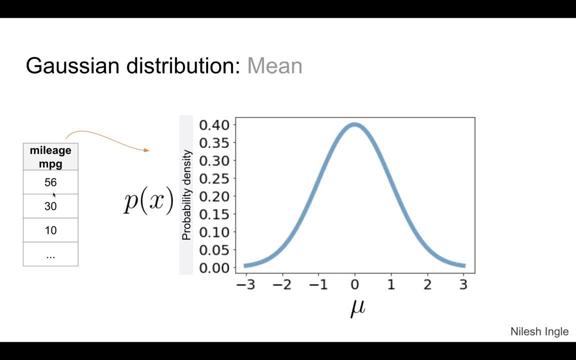 look at our data set of my miles per gallon mileage. we can plot it in this form where we have a Gaussian curve. in real world the miles per gallon may not look like this, but for sake of this video, let's assume that the distribution looks like this and we have normalized values on the x-axis, which is: 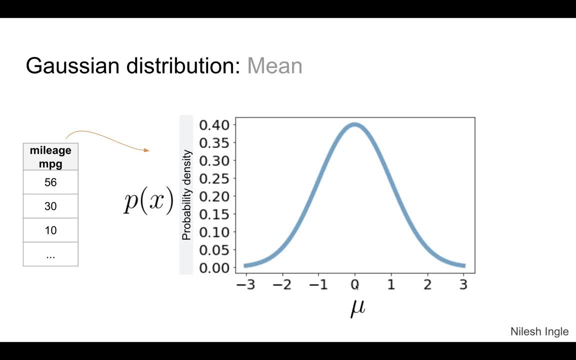 the miles per gallon and the zero indicates the mean. so the center in this case is mean, because this is a well-balanced symmetric curve, which is the normal distribution, and on the y-axis we have the probability density. and the reason why we are discussing this plot is because the entire discussion on 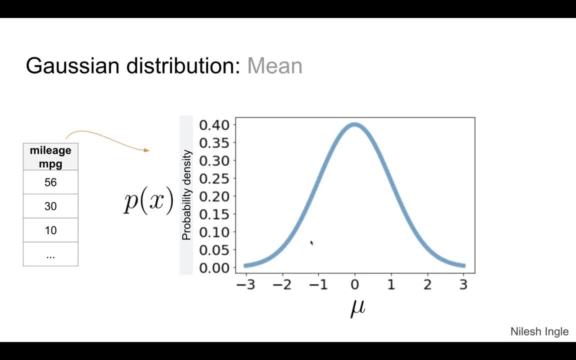 Gaussian mixture models depends on understanding this particular plot. right here we'll be talking about these probabilities that the densities that are on the y-axis and the mean and the spread of these uh curves so spread. I mean the standard deviation. so if you are one standard deviation away from the mean, this is the region. if you are two, 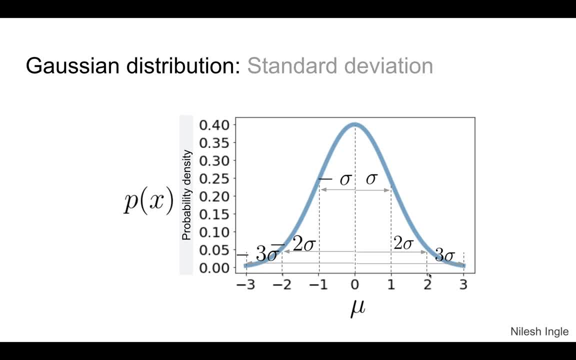 standard deviations on the positive side. this would be the distance three standard divisions is up to here, and similarly we have the series change of that. you can see that the hardness or частоness of the curve depends on range or more than one r, but there's a few. possible ways to show. if the null dynamics are the norm, this will be loopholes waiting for spot the. of course, going to the corresponding basis of weins and rounds and ainionglass means that that top of the curve is now in the quotation marks, that the dashed edge goes over the top. 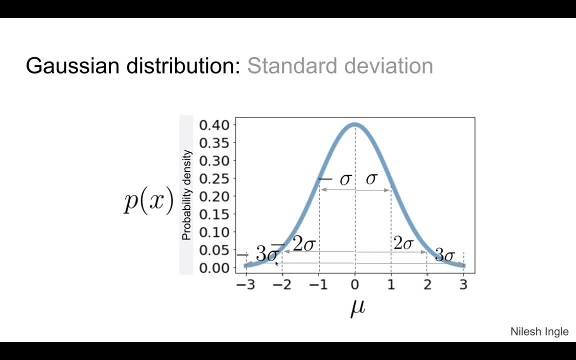 half Theунд reinforces about once, and i mean unless we are at simplesmente subtracting the The Huh. similarly we have the same one, two and three standard division on the negative side of the mean. so we would use these: the mean, the variation for each of the features or each of the data. 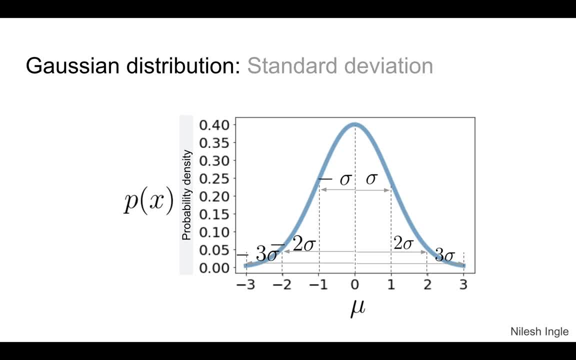 points to find out how close or far they are from either the center of the cluster or the the mostly from the center of the cluster, and so that would help us make a decision whether that point should belong to a specific cluster or it should belong to a 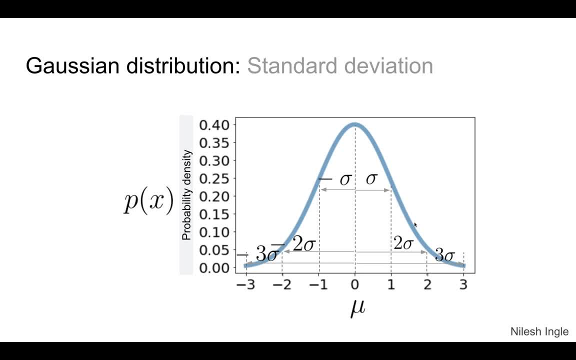 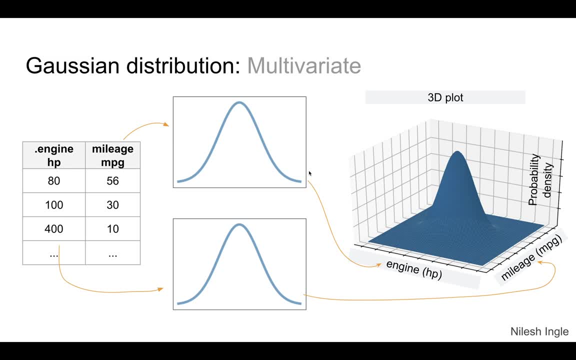 different cluster, and this is for just a single variable. we are looking at now if we have two or more variables, that would be multi-variate. so for two variables you'd say it's a bi-variable. and here we have two features now: engine horsepower and miles per gallon. 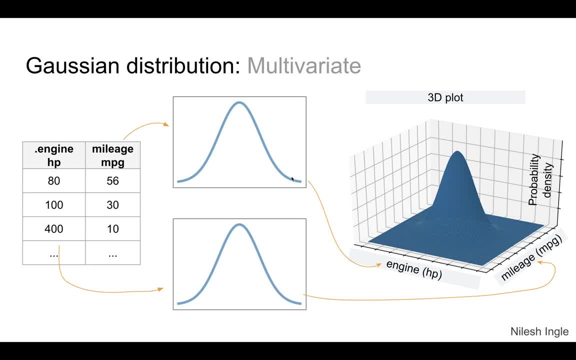 and let's say, the two curves look like this. they are gaussian. and when we try to plot them we see a 3d plot, as shown here. we have engine horsepower, miles per gallon on the x-axis. on the z-axis we have the probability density. now how do we read this plot? so this is: 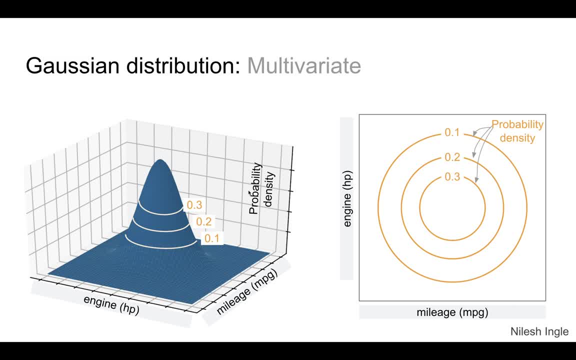 the method, and you'll see these types of plots in several times now in this video, and so it's important to know how to read this. if you already know how to read them, you could skip this part. basically, what we have is in this particular surface plot. these rings represent, let's say, the 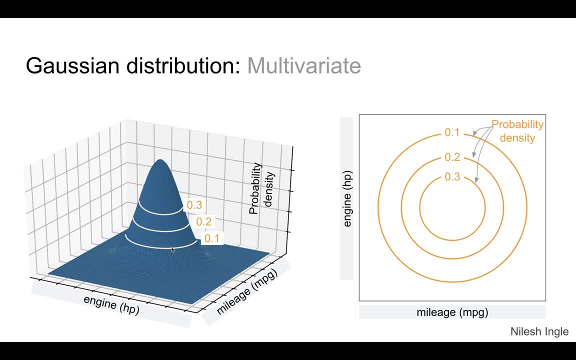 levels or hurricane scales or Đây Hay gold or on Block线. height of the data points from the floor. of this plot, so the bottom most ring is at 0.1 height from the floor. so that's the 0.1 probability density, then the next one is 0.2, then 0.3. 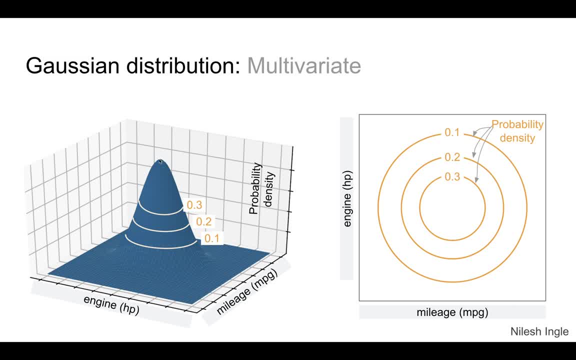 and as we go up to the top, that would be the maximum value and we can represent. instead of looking at a 3D plot, it's easier sometimes to look at 2D representation of this 3D plot, which is shown on the right hand side, and the name for this type of plot is contour plots and in this 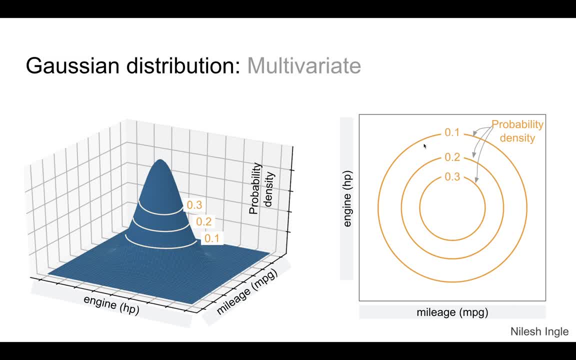 plot. we have the same ring, so 0.1 is the larger ring because it's at the towards the bottom of that surface plot and we have the same length and width of that surface plot, So that's the number of contour plots. So we have 0.1 height from the floor to the floor and we have the number of 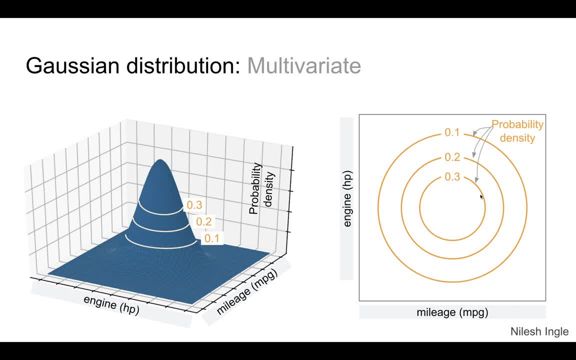 0.3. that's in the center. that represents the higher value for the probability density. so this is like a mountain and think of it as a mount. looking at a mountain from the top and on the points on this ring would have the same value. so the outermost ring, anywhere on that ring would. 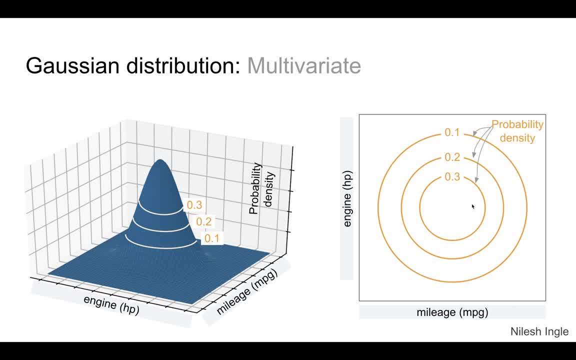 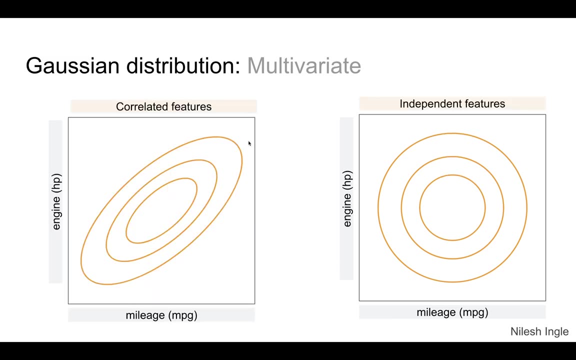 have the value of 0.1 and so on for the other data points in other rings, and here, as we'll see, the shape of these contour plots also make a huge difference. so if the plots are oval in shape, as shown in the left hand side, it tells us that there is some interaction going on between the two. 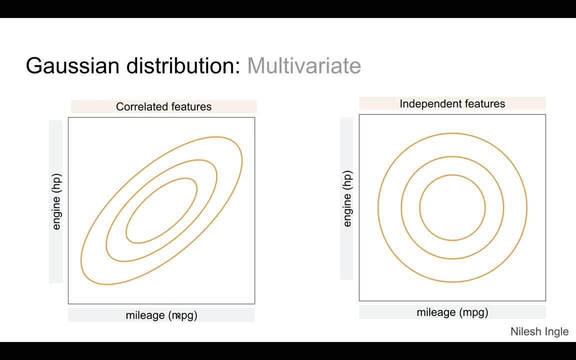 features here: engine, how, how and miles per gallon. maybe if the the curve actually, if you think about it, practically doesn't make sense, because as the engine horsepower increases, the miles per gallon should drop. so maybe though i should have drawn the oval this way. but anyways, there the oval shape. 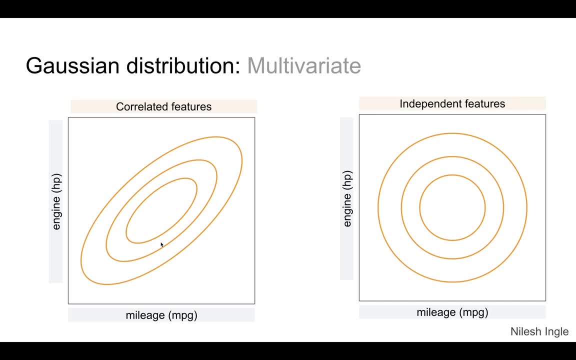 does indicate that there is some interaction, so the features could be correlated to a certain degree. however, on the right hand side, we can see that the contours are circular. it's a perfect circle, which suggests that there is no interaction between the features, engine and the mileage, and so the features could be considered as independent now in mathematical terms. notice that.